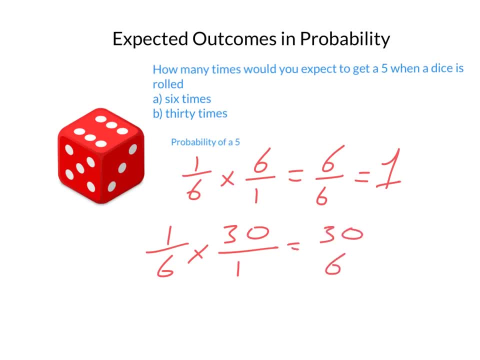 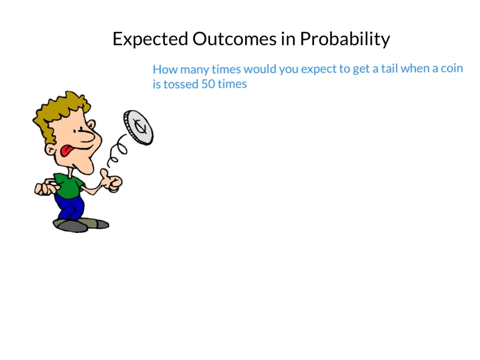 30.. Six times one is six and of course we always try to simplify our fraction: 30 divided by six equals five. So if the dice was rolled 30 times, you could expect to get a five, five of those times. Here's another question: how many times would you expect to get a tail? 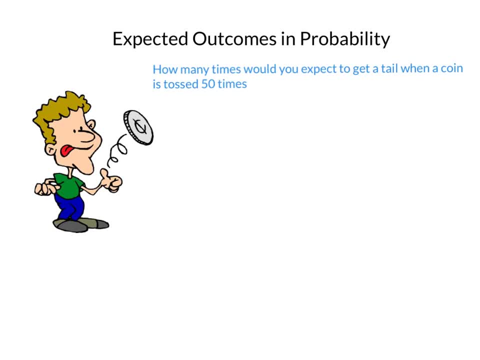 when a coin is tossed 50 times. Well, the chances of getting a tail is 50, 50 or a one in two chance. So we simply multiply that by 50 and 50 times a half is 25 times. So you would expect to get 25 tails if a coin was tossed 50 times. 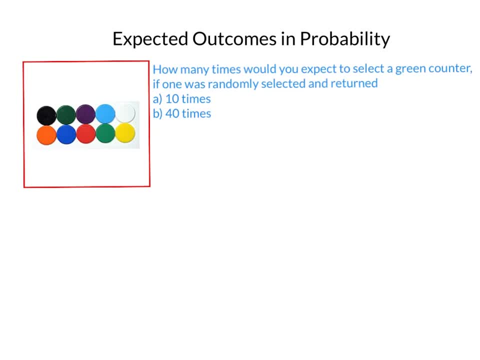 And finally, how many times would you expect to select a green counter if one was randomly selected and returned a and 10 times, b, 40 times? Well, there are two green counters out of ten counters in these boards: 8, 10,, 20,, 40,, 50,, 33,, 45 times. 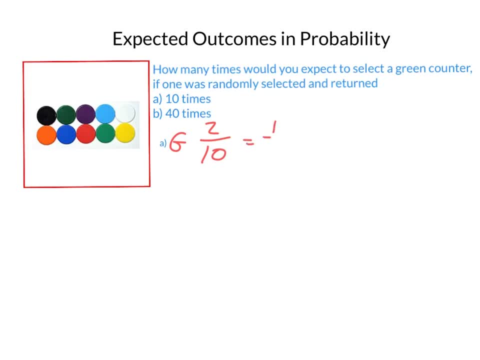 altogether, which is a 1 in 5 probability of choosing a green. and then, if we did this 10 times, we simply multiply by 10, which gives us 10 over 5, which simplifies down to 2. so if the experiment was done 10 times, you could expect to get the 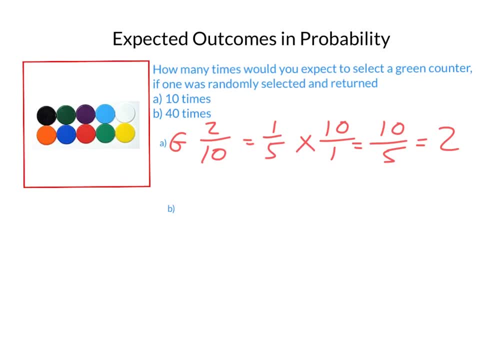 green twice, and if the experiment was done 40 times, well, again, our probability of getting a green was 1 in 5. so this time we simply multiply it by 40. multiplying the top by the top gives us 40 on the top and 5 on the bottom. 40. 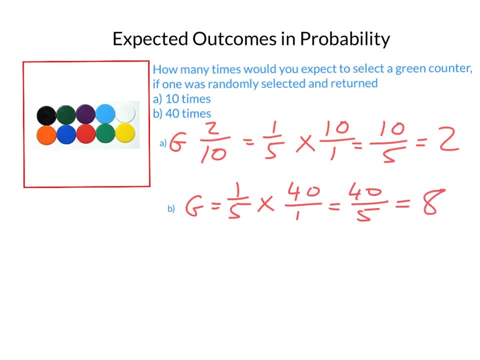 divided by 5 is 8. so if the experiment was done 40 times, we simply multiply by 10, and if the experiment was done 40 times, you could expect to choose the green 8 times.